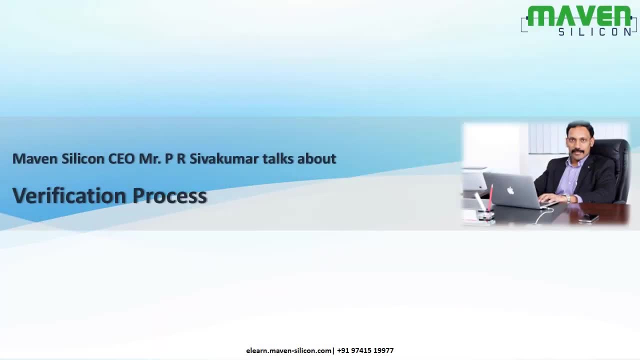 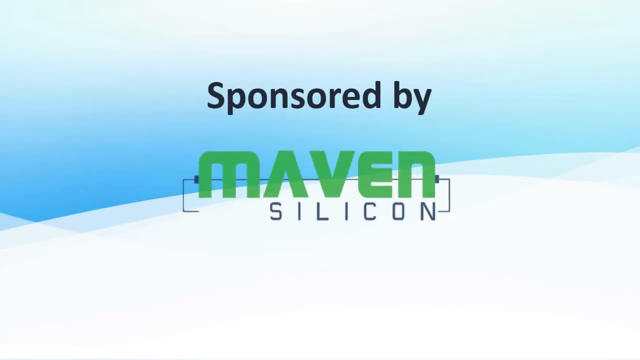 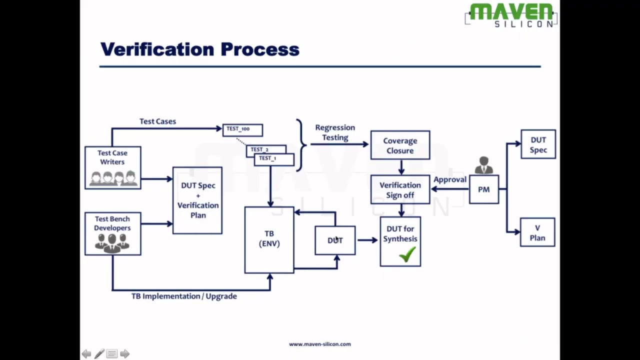 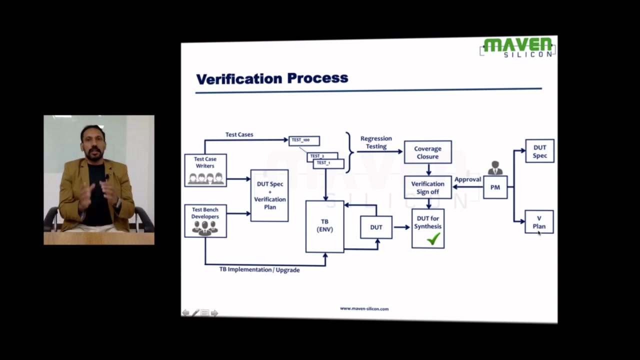 Okay. so now let's look at the entire verification process: Project Manager: He wants the complete verification. He takes the design specification and defines the verification plan. So even if you are going to be a junior engineer, you need to know how to define verification plan. Once you understand the verification plan, then 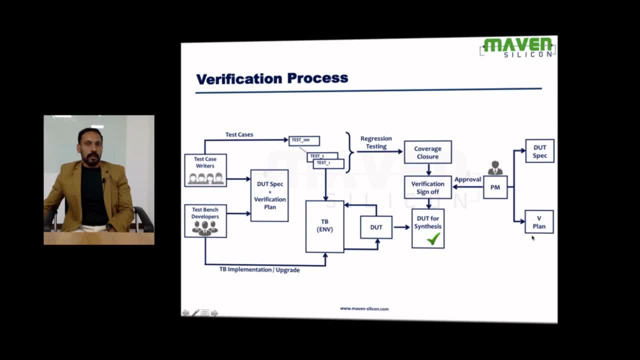 you would be able to deal with it. But when you work with any company, there is a person called Project Manager and he is the person who is going to define the verification plan. If you look at verification plan, basically it defines everything: The test bench, architecture. 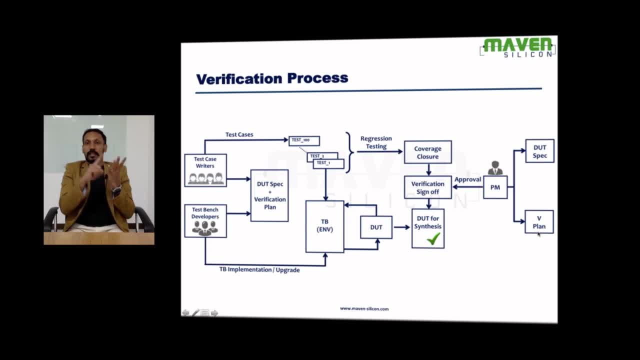 coverage model, self-checking strategy, the test cases, the scenarios, everything will be captured in verification plan And he is going to take care of the coverage, closure and verification site And then he is going to sign off when the design has to be released for synthesis. 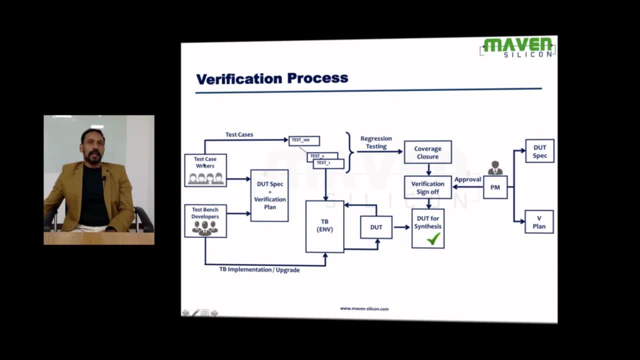 So basically, there are two teams. One is the test case writers. The other one is test bench developer: Experienced engineers- engineers with three to five years experience. they own the test bench design. They make use of the language features. languages like system. 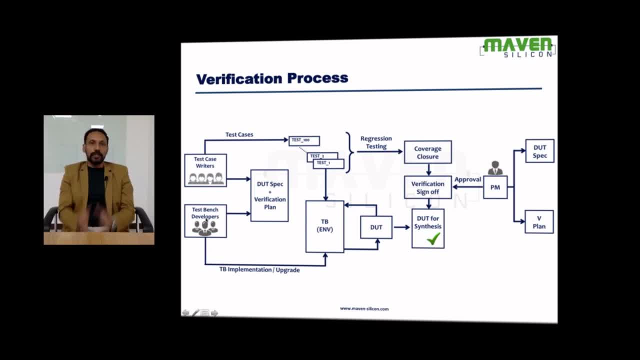 Verilog and implement the test bench. And junior engineers who don't have much experience with the test bench design: they want to implement the test bench design. And junior engineers who don't have much experience with the test bench design: they want to implement the test. 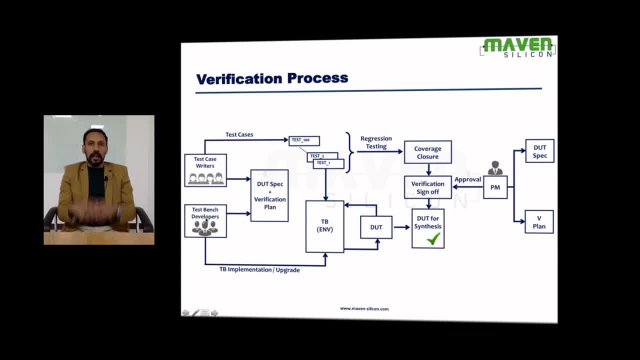 bench design And junior engineers who don't have much experience with the test bench design. they want to implement the test bench design. And junior engineers who don't have much experience. they write test cases, They run the test cases and generate coverage. Look at this Test. 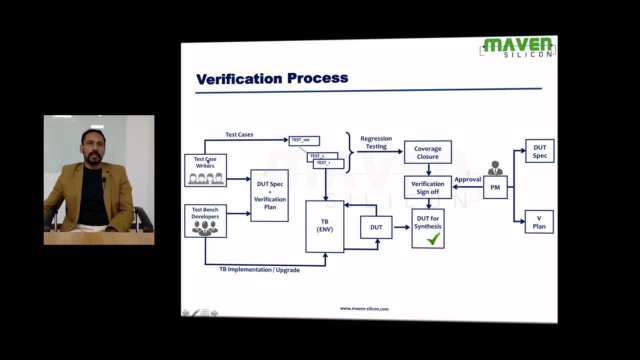 case writer And both the teams, test case writers and test bench developers. they refer DUT specification and verification plan, The plan which is created by project manager. So when it comes to test bench- basically these people- they need to understand the test bench architecture. 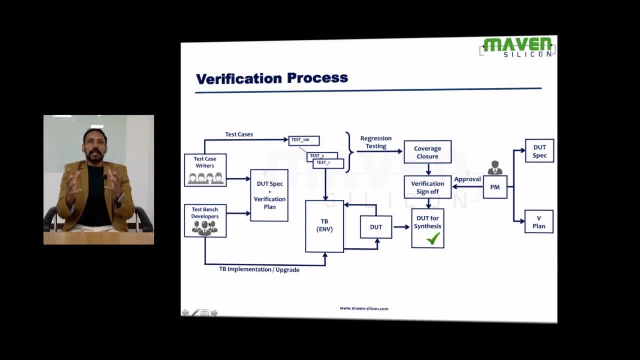 How they can implement the test bench: How many drivers, How many generators, How many monitors, What kind of scoreboard, What kind of coverage model. They have to follow the test bench architecture to implement the test bench At the same time, the test case. 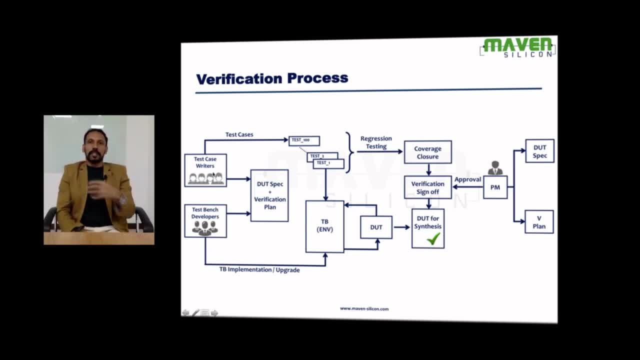 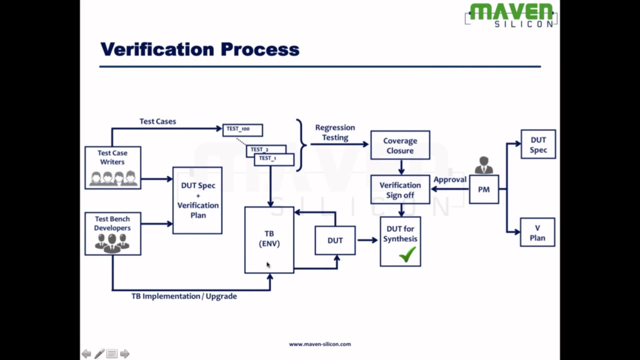 writers. they are going to look at the scenarios, What kind of scenarios basically they have to generate And what is the coverage goal, How many test cases they have to create. That's what they are going to look at. So both the teams they will refer. DUT specification and verification plan: Test bench developers. 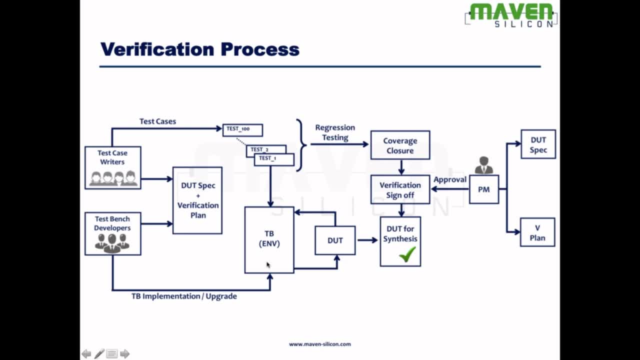 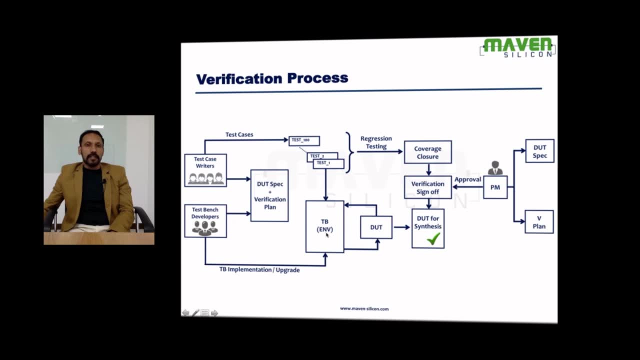 write some basic test cases and run simulation. They make sure that the data flow happens properly within test bench. So what they do is they instantiate the design within test bench and they make sure that the data flow happens properly And, after creating the complete setup, they hand over the simulation environment to the 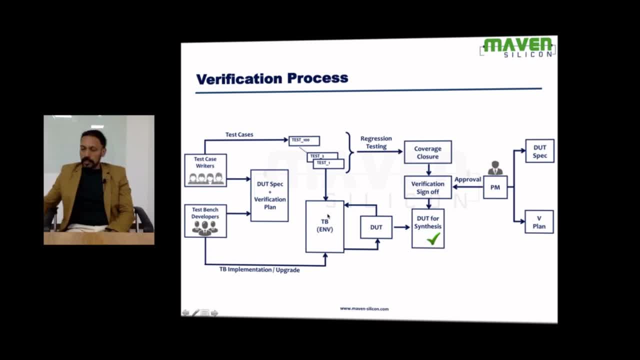 test case writers, Then the test case writers. they will write different kinds of test cases, like hundreds of test cases or thousands of test cases, And they will run the test cases one by one. They make sure that the design works in all kinds of scenarios. So basically, 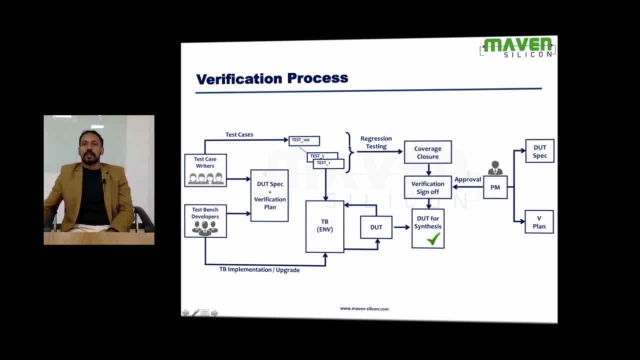 the test case writers own the complete regression testing, So every time when they run test case, they also generate coverage. And finally, what they are going to do is they are going to merge all the coverage data, different kinds of coverage, information like code coverage and functional coverage, And 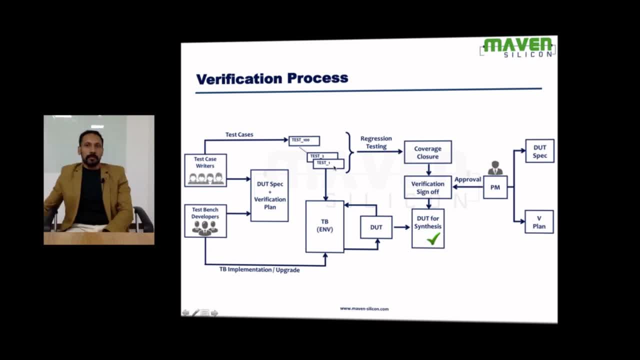 then, finally, they are going to merge all the coverage information and they are going to generate the final coverage report. Eventually, the project manager is going to look at the coverage report and if he's going to be happy like okay, 100% coverage, then he will sign. 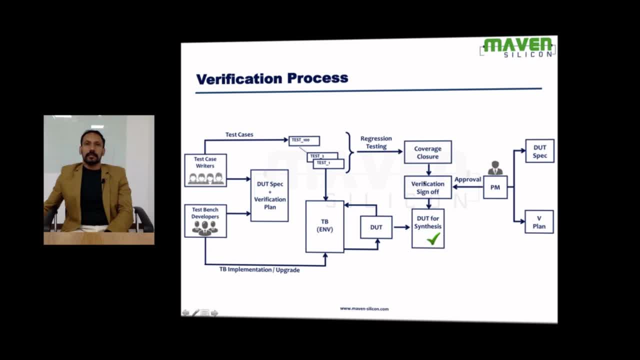 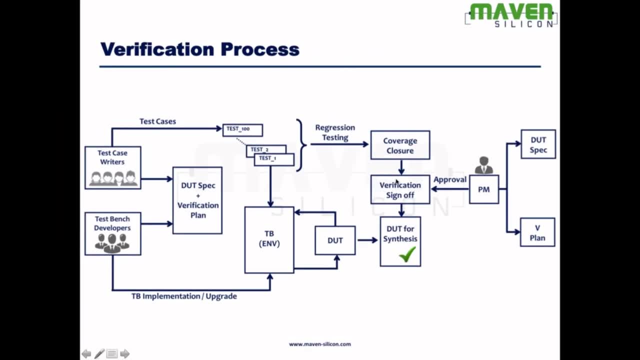 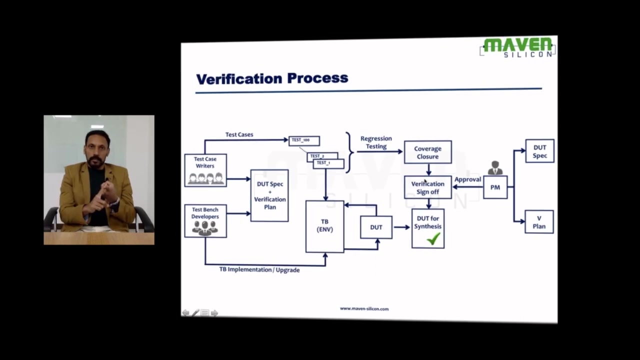 off the simulation, Then he would say: the design is ready for synthesis. That's how the sign off happens. This is how, basically, the verification happens. Now, to be part of the simulation process, you need to be good at various things. You need to understand the test bench implementation. For that you have to improve your programming.